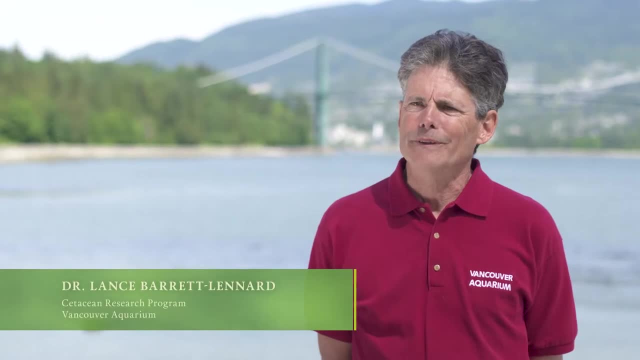 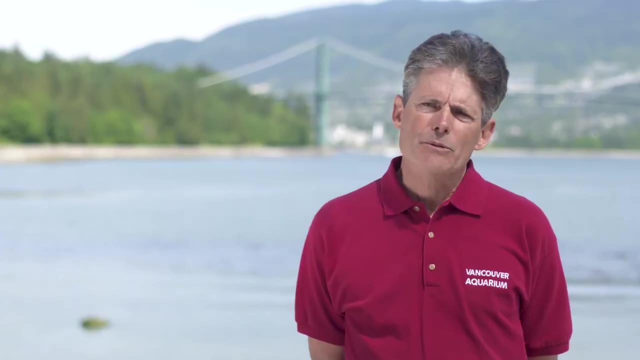 Killer whales are an iconic species of animal Around the world. people are just incredibly interested and attracted to the species, And here in the Pacific Northwest we're lucky enough to be in a place where we can see them swing by quite often. We know that if they're 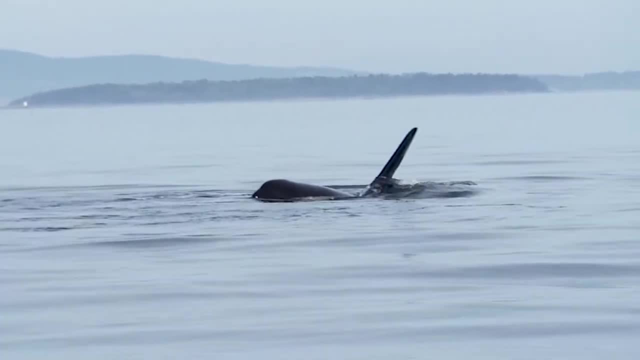 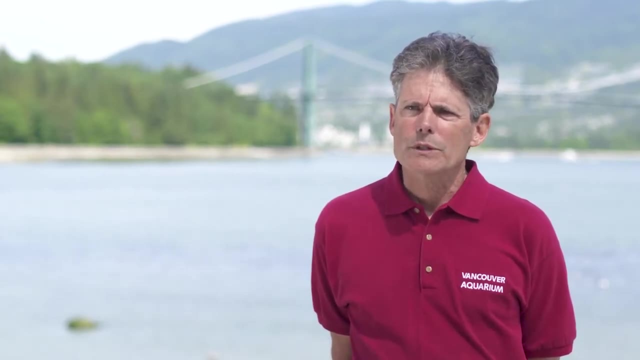 having difficulty. they're affected by human activities in many ways. I can't overemphasize how critical the situation is right now for the southern resident killer whales. Only 78 animals, lots and lots of challenges, But on the positive side we've got a research. 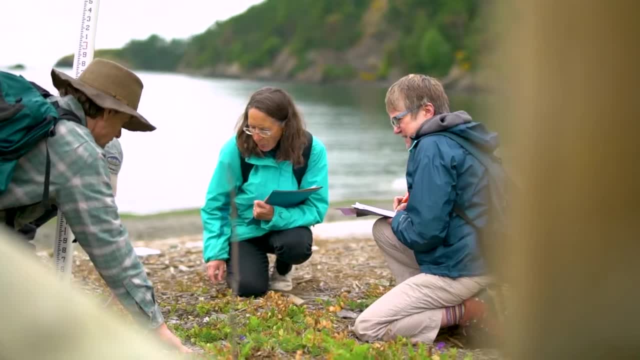 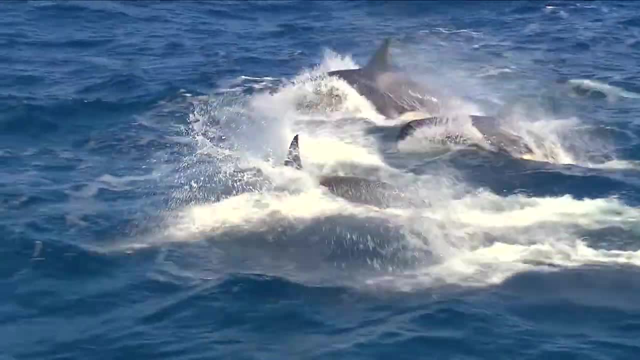 community that's very motivated and well-equipped now to tackle a lot of the problems and understand them better. So there's a lot of positive momentum. at this particular point in time, The National Fish and Wildlife Foundation, in partnership with SeaWorld Shell Oil Company. 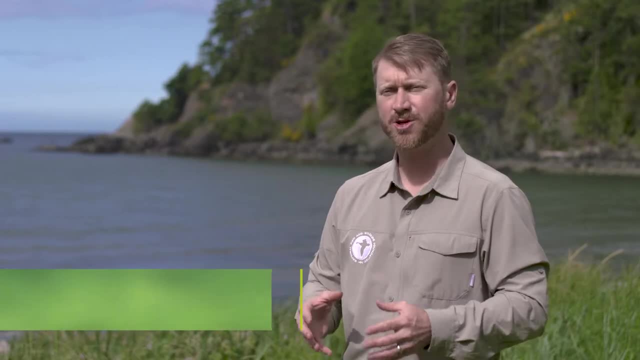 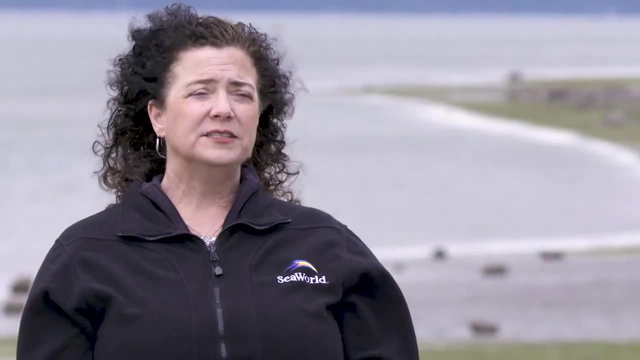 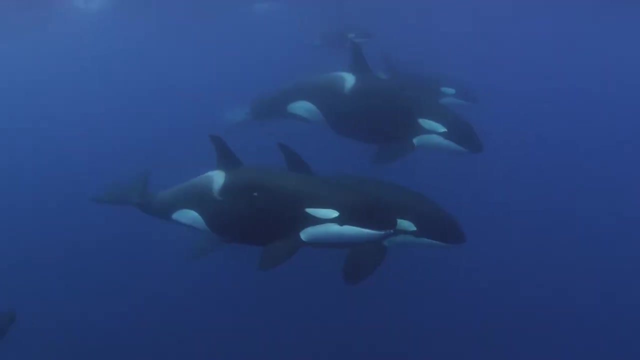 the US Fish and Wildlife Service and NOAA are funding grants in strategic areas in order to aid and recover. Our job at SeaWorld is about much more than just introducing the population to killer whales. We really are concerned about what's happening with these populations in the wild. 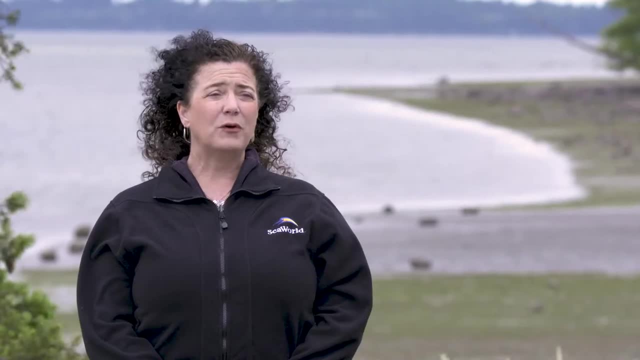 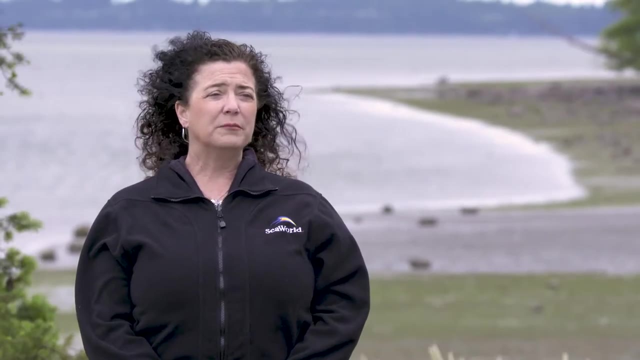 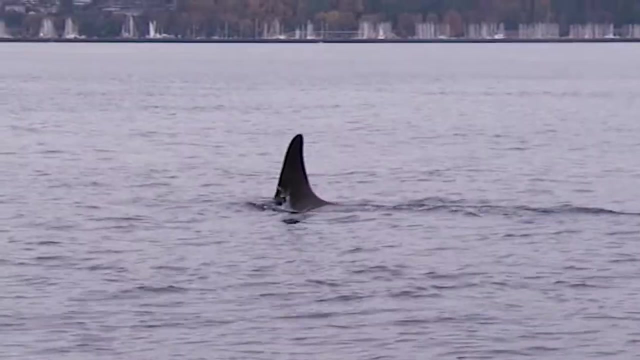 Because of that, we partner with conservation organizations as well as biologists and researchers throughout the world, but especially in the Pacific Northwest, to look at ways that we can improve the lives of the killer whales that live there. The work that we're doing today may seem unrelated, but all of these projects come 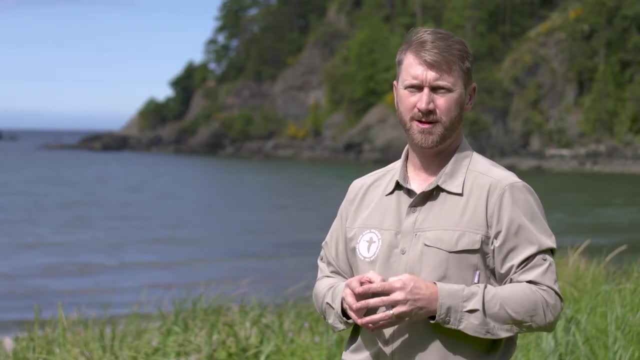 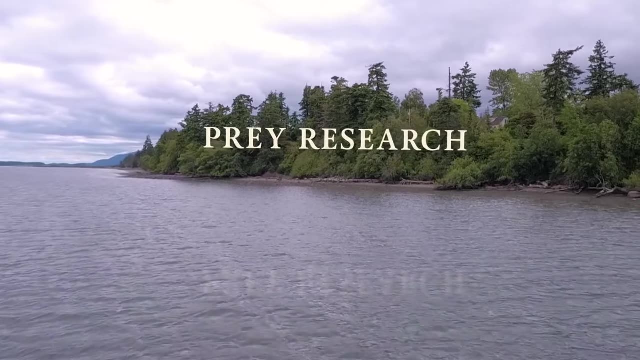 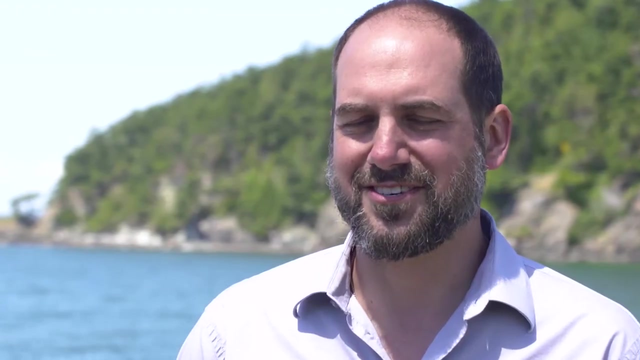 together to aid in one thing: to increase the populations of Chinook salmon, the number one prey species for the killer whales. Chinook populations have declined up to tenfold in the Salish Sea. This is a serious problem for killer whales because their diet consists of over 80 percent of Chinook from this region. 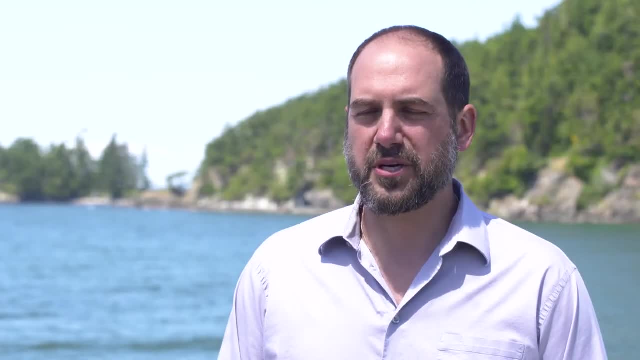 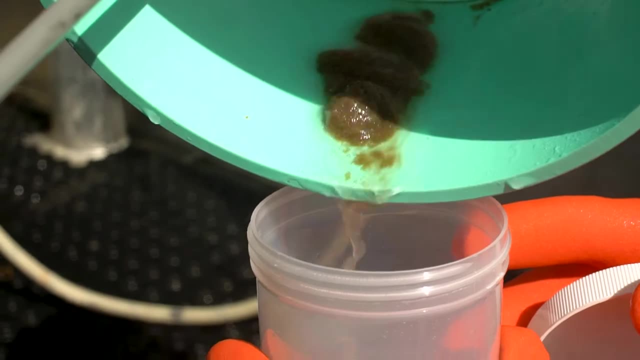 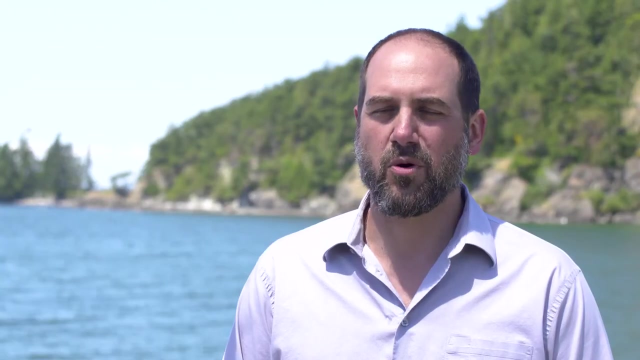 in the summer. We've found strong correlations between the community structure of zooplankton and salmon survival. Understanding zooplankton is important to getting a handle on what is driving the survival of salmon. We're working towards a future with more salmon and thus more prey for killer. 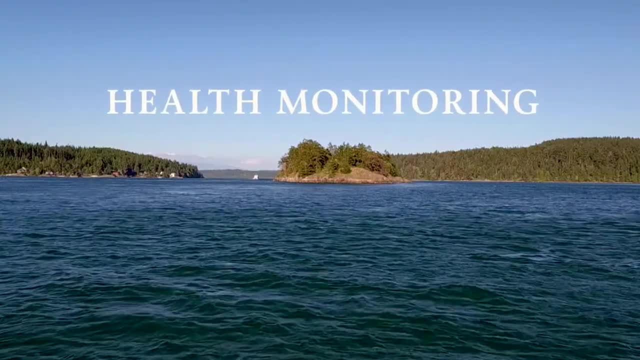 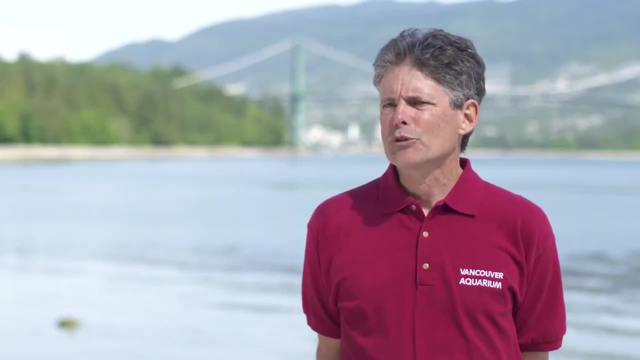 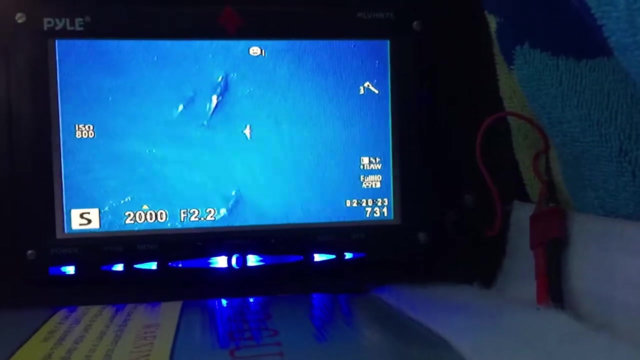 whales. Before we started the photogrammetry work, the only way we could tell how killer whales were responding to shortages in food was by counting the mortalities. really Looking at them from above gives us an entirely different perspective. We can see how widely they're.